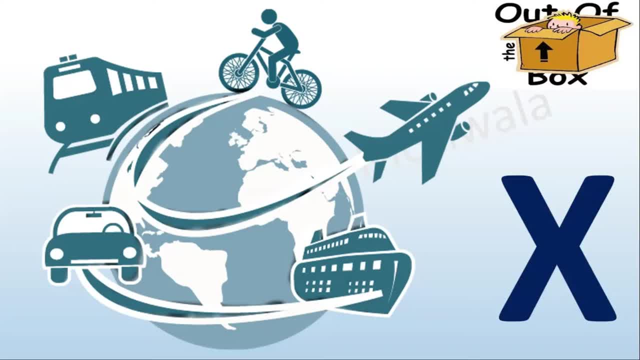 no relevance to this topic is of no relevance to this topic, whatever means of transport they use. we are not interested in that. Then the question will be what we are interested in. if we are not interested in modes of transport, in transportation, then what we are interested in, the thing which we 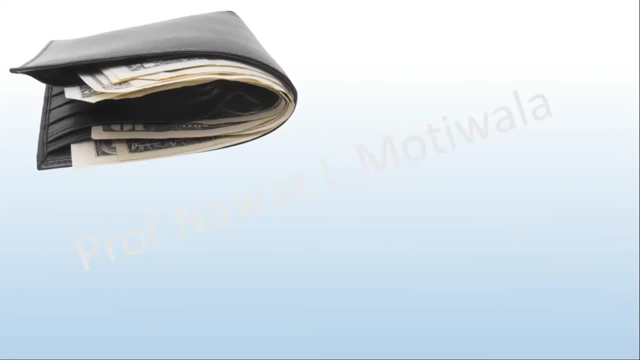 are interested in is paisa. What will be the minimum cost? We have to talk about everything in terms of money: Where will it take less money and where will it save more in our pocket? So that is the aim of this topic, This entire chapter. we want to find out what will be the total optimum transportation. 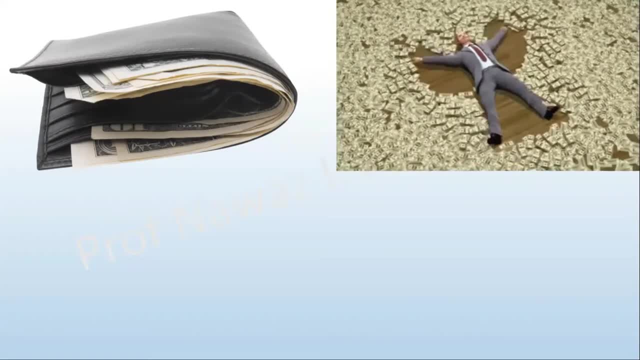 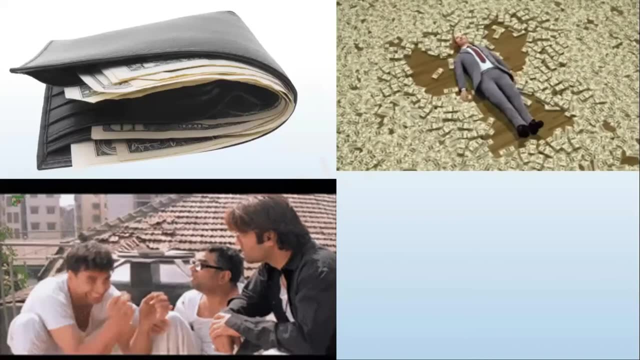 cost. We want things around us like this, and this will be only possible when we reduce the cost, which is anchoring. and to achieve this kind of case shortcut is this one where you will be having a lottery and then you enjoy. But as a technical person, we will not rely on this type of things. 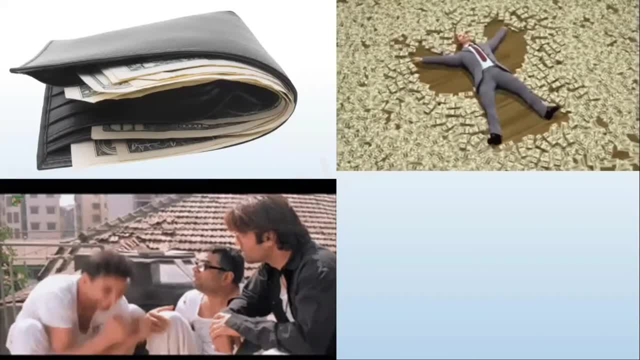 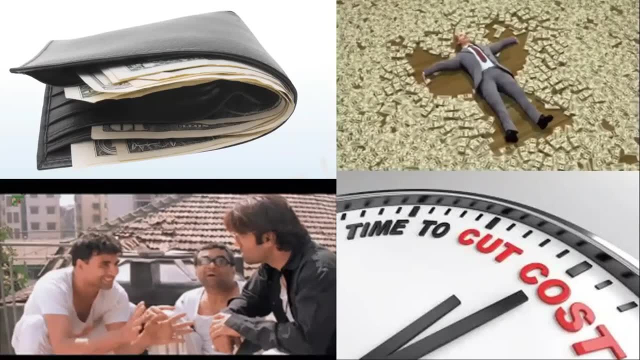 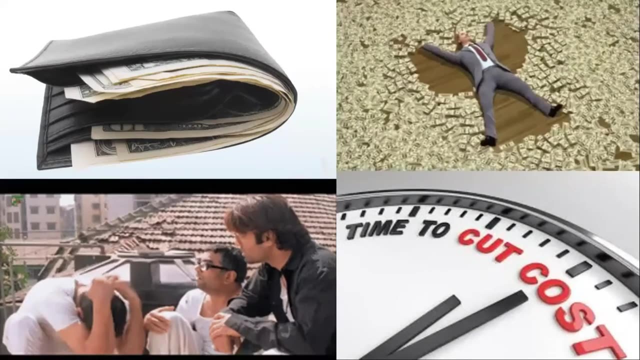 We will say, technically, how can we reduce the cost? It is now time to cut the cost. So we will not rely on any lottery or something to get our things done. We will apply our engineering mind or technical mind and cut the cost which is going to be incurred. and as we cut the cost, 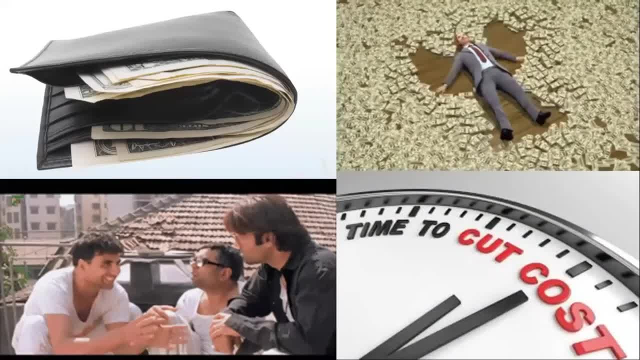 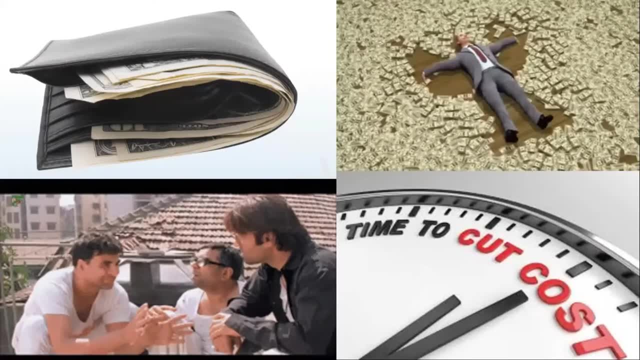 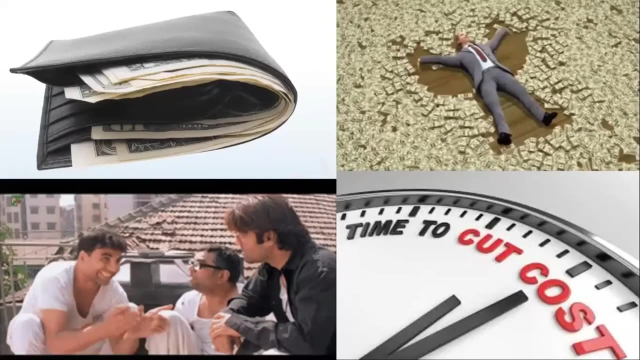 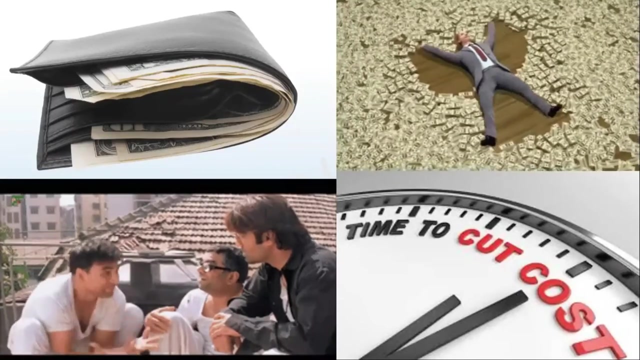 the same cost will be coming into our pockets as our profit. So the entire aim, the entire aim of this chapter is: what would be the minimum transportation cost to meet the necessary demands and from various supply sources. What would be the minimum transportation cost? This is the objective of this entire chapter. 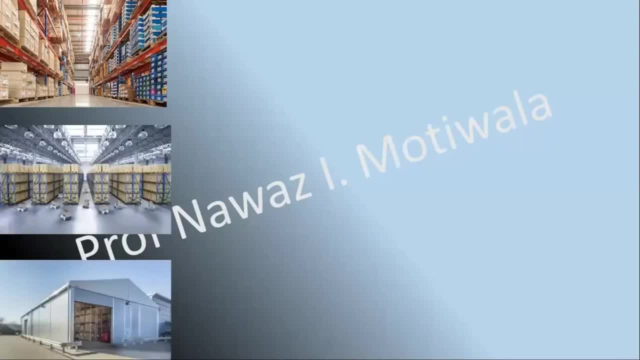 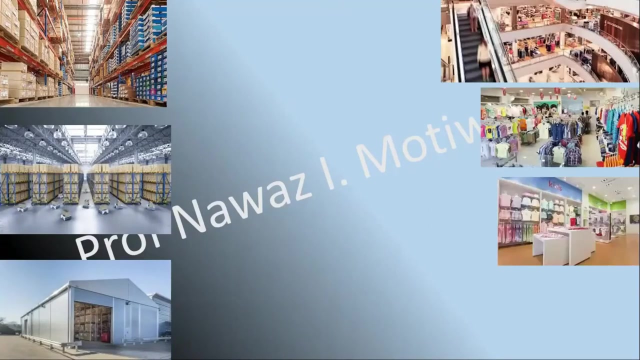 Let us say there is a firm who has three different warehouses. These are the warehouses where they store their products, and these three are located at different different places. Let us say one is located in Chennai, one in Bangalore and one in Mumbai and they have to transport their material. 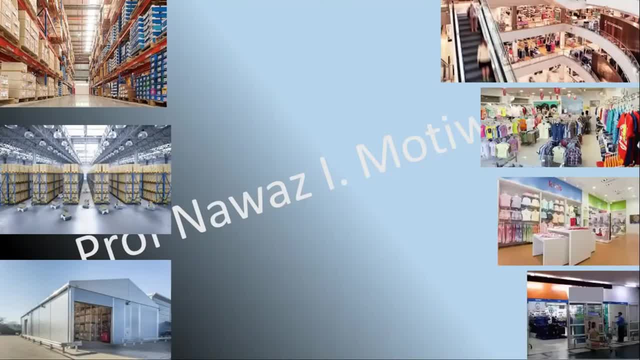 to these four different locations. So on the left hand side you can see there are three storage places, or I can say the supply points, and on the right hand side it is the demand points. Demand points means where these products will be sold. So now it is the aim to transport this material. 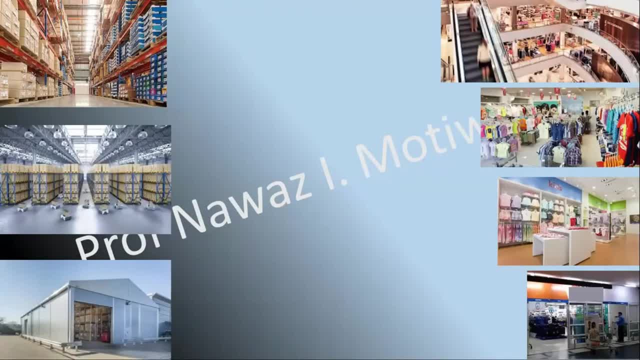 from supply point to demand point, From wherever our material is kept, we have to transport it from wherever it is required to be transported. So to transport this, from which point it is going to be transferred from. So to transport this from where the material is kept. So to transport it from where. 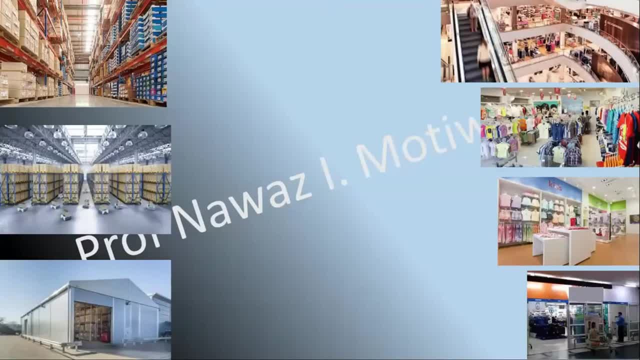 of the supply point to which of the demand point i will supply- this is my main question- such that the total transportation cost should be minimum. so let me explain with a sample. let us say there is a tempo service and i have to transport all these items from my warehouse to my demand points. 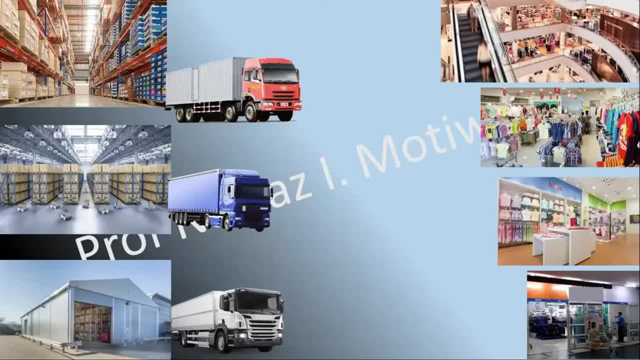 and demand points are again located at various places. so now my aim is how i can transfer this products from my supply point to the demand points. so it can be one of the way, let us say, warehouse one, warehouse one- can supply to all the four demand points. similarly, second warehouse can. 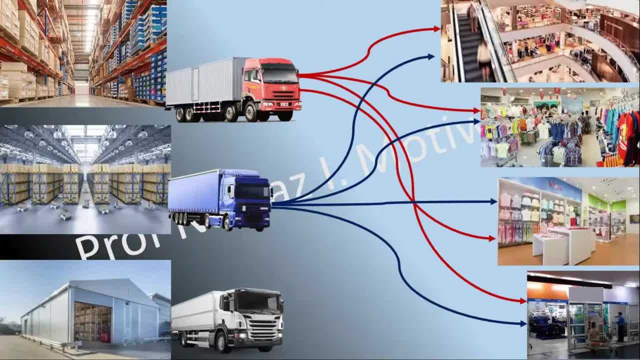 supply to all the four demand points, and similarly, the third warehouse can also supply to all the four demand points. so these are the possible cases. now let us see the cost incurred with each of this. as it is mentioned, if the commodity is transferable from warehouse one to demand point one, the cost associated, or the transportation cost, will be rupees. 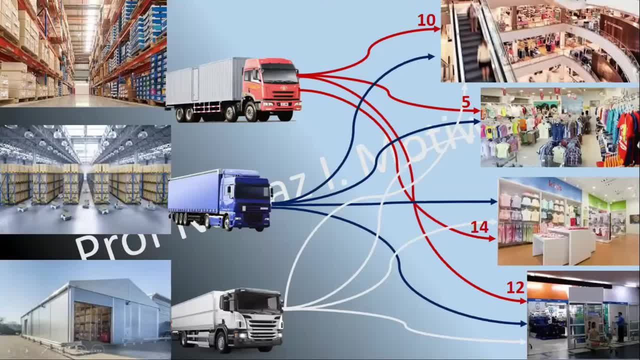 10 per unit, the transportation cost will be 10 per unit of all the units that will be transported. similarly, if i transport from the first point to the second point, the cost incurred to me will be five rupees per product. similarly, this is 14 and this is 12.. now, if i show you only this pick, 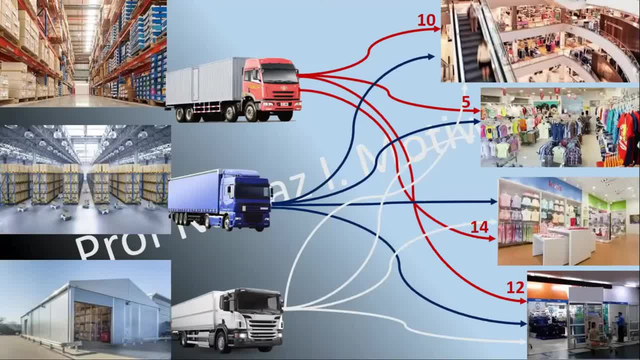 so you will say, sir, it is simple. directly, the first will go to the second demand point, because the transportation cost associated with it is five. it is minimum of all these three. so i will transport all the commodities from warehouse one to demand point two. okay, now let me proceed further with the 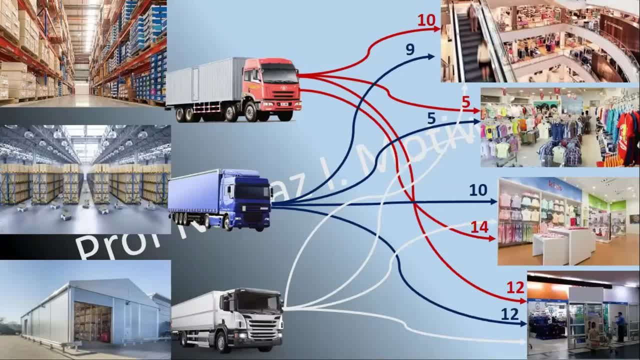 values of other points. now let us say these are the values wherein the cost are from warehouse to to the demand. various demand points. if i supply from first supply point to the first demand point, it will be 9 rupees. similarly, from second supply point to second demand point, the cost incurred will be 5 and. 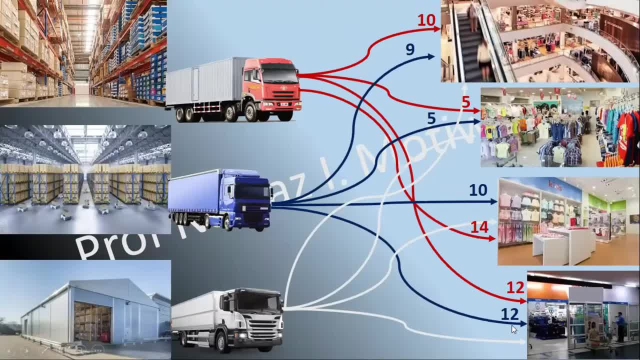 third, 10 and fourth, 12. now there is a confusion in your mind. first it was very clear that yes, as the cost was rupees 5, only from warehouse 1, it should be supplied to demand point 2. but now I gave you one more option that the cost. 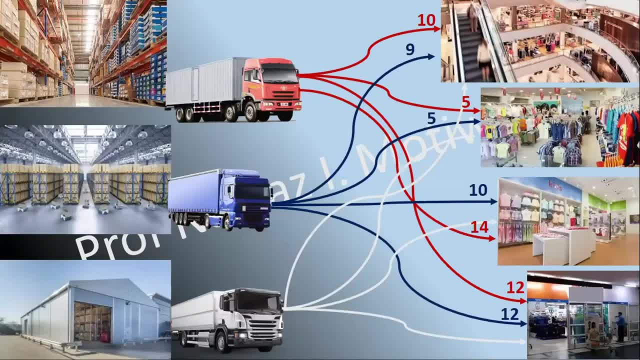 associated with second warehouse and second demand supply point is also 5. so what you will say now? you will again say: yes, sir, you can supply to the demand point to either from 1 or 2 ticket. now your conclusion will be: supply to demand point 2 from warehouse 1 and warehouse 2. 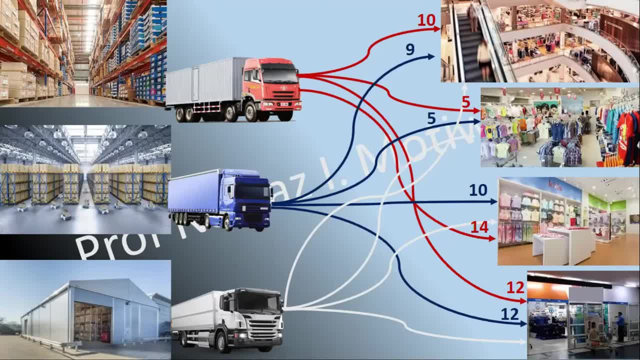 similarly so it is not the case for both of them. you are giving it to demand point 2 only, so what will be the other demand points doing? there will be lack of supply there. now let me extend this further from the third warehouse to various demand points. the cost are like this: okay, the cost are if I supply from 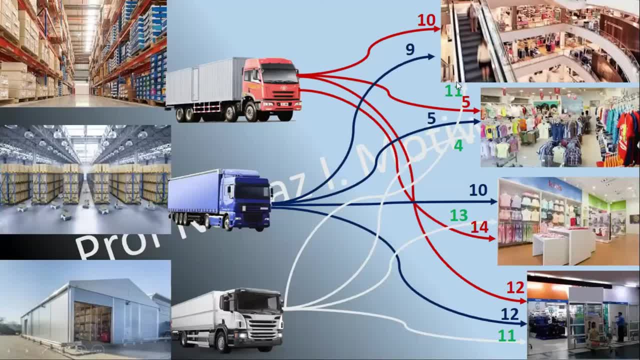 third warehouse to first warehouse cost of supply will be 11 rupees per product, here it is 13, here it is 11 and here it is 4. so again we'll say: sir, the supply cost from third warehouse to second warehouse is again me minimum. hence we will supply to from warehouse 3 to demand point 2 as minimum. 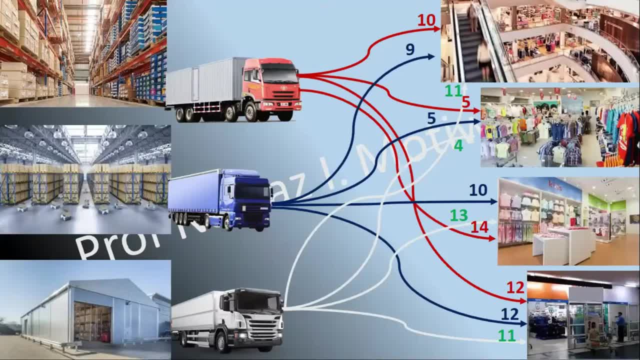 cost is 4 of demand point 2 from warehouse 3. we will supply to it. then next is 5, but 5 already demand 2 pe hai, jo already fulfill ho chuki hai, so hum usko nahi dekhenge. next kya hai minimum cost? next minimum cost is 9, so 9, you can see 9 is. 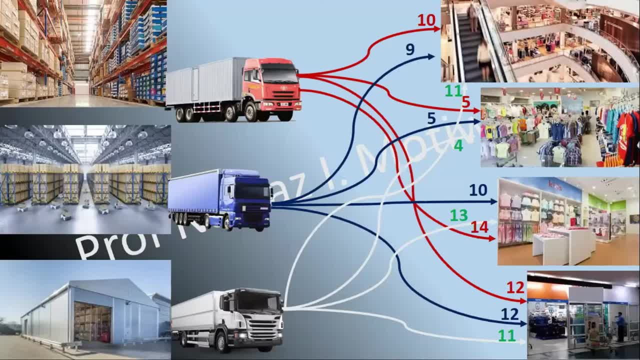 the cost associated from warehouse 2 to demand point 1. ab kya ho gaya, demand point 1 bhi satisfied ho gaya, usko bhi maal mil gaya from warehouse 2. next thread: 10 ab 10 hai from warehouse 2 it can go to demand point 3 or from warehouse. 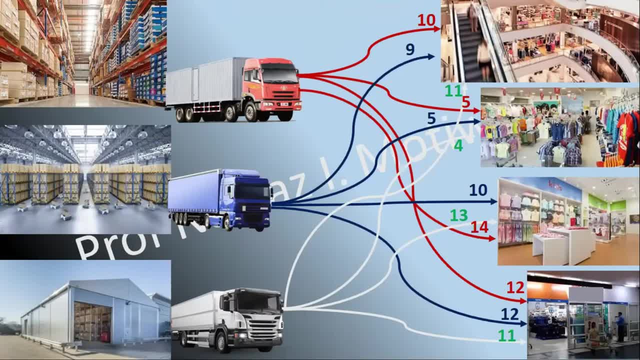 1. it can go to demand point 1. ab yaha par fir se confusion, konsa kisko bheje. so the point which I want to make you understand is it will be very difficult and tedious task to find out which from which warehouse 2 which demand point. the component should be shipped such that: 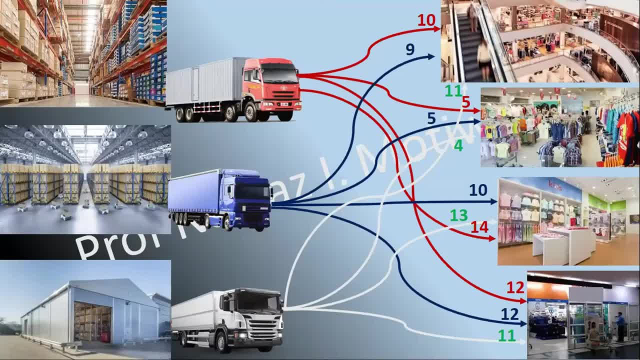 transportation cost is minimum ab ye toh ho gaya sip itti baat isme tum log phas gaya kya konsa kaha jaega ab me uske andar aur constraint dal raha ho. the constraints are like this. observe on the pics. the values are 100, 100 and 100. what are these values? this? 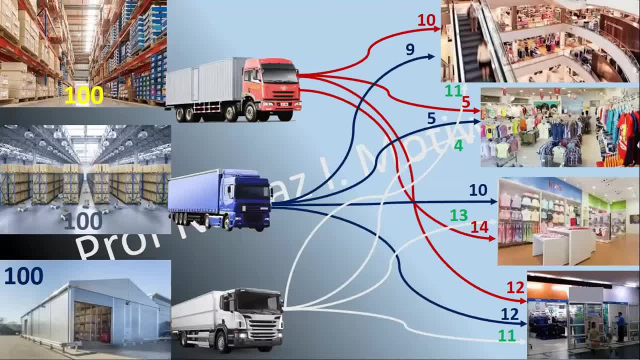 values are: the warehouse 1, warehouse 2 and warehouse 3 can supply only 100 products, unke stocking with that of this hundred, maybe hundred tons, anything, we just emphasize on the number. the warehouse one, warehouse two and warehouse three can supply only hundred products each. and now let us see demand points. the 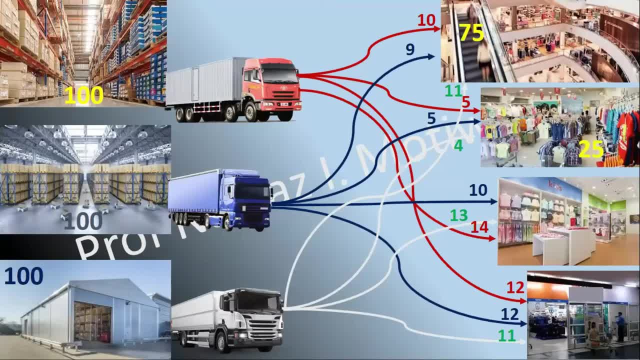 demands here are 75, 25, 120 and 80. okay, so these are the demands at the particular different locations. now it goes into more complexity if I a top cost me, I'm passing right there after the supply demand is earlier. I will be check Karna up, yeah, but just observe this one. the second one, the cost, are 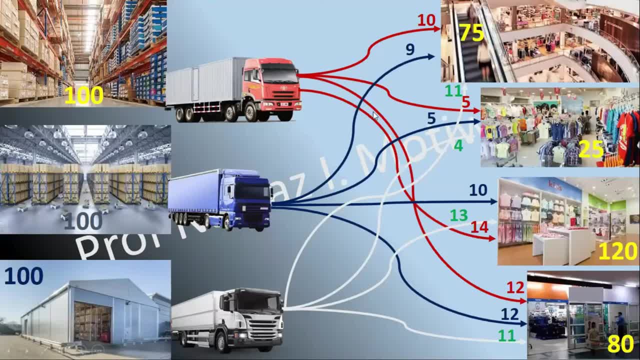 lowest if I supply it from warehouse one to demand point two, it is five rupees. from two to this point, again it is five. from three to this point, again it is four. the cost is minimum. so you will say that supply from all this you can supply. 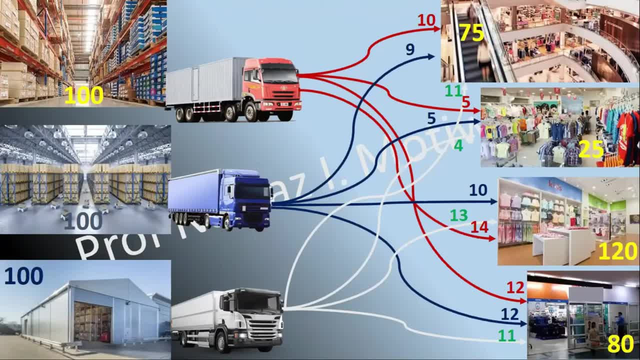 from all this. but there is no demand there. demand in a supply, there is demand of only 25 units. so let us say I have fulfilled days demand of 25 rupees from the mean minimum cost. that is fourth. so for many warehouse 3 said demand to cost sub. 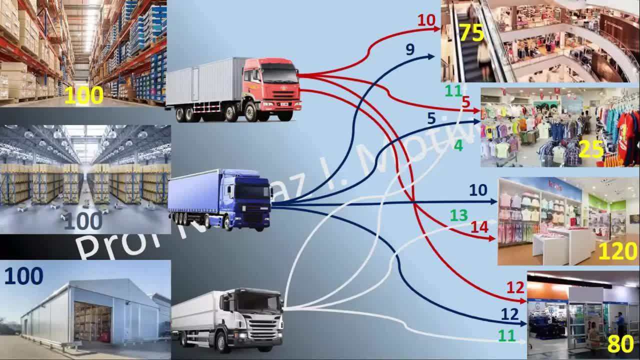 Adam Korea up. it is irrelevant of the cost of will suck sag. it's our, our show. it is irrelevant of cost up it not be just a poi demand toNTm, which a requirement in a year, but demand at that warehouse is already fulfilled. i have to check what is the demand at the demand end and 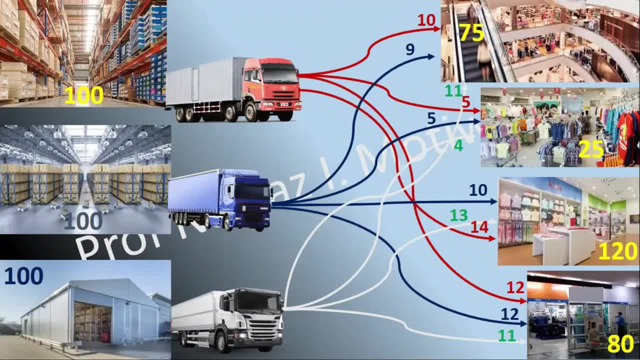 how much i can supply from each particular warehouse such that all the demands are met and the transportation cost is minimum. so, after explaining all this, to summarize this, this slide it is- we need to find out the minimum transportation cost such that it will fulfill all the demands from various supply points. 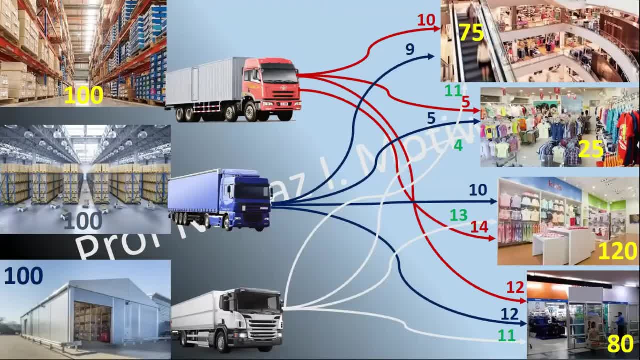 such that all the demands are fulfilled from the respective warehouse points, whatever it is possible. so this is the entire thing which we have to find out in this particular topic. so you have seen that if we go by regular method of thinking, then we will be into more. 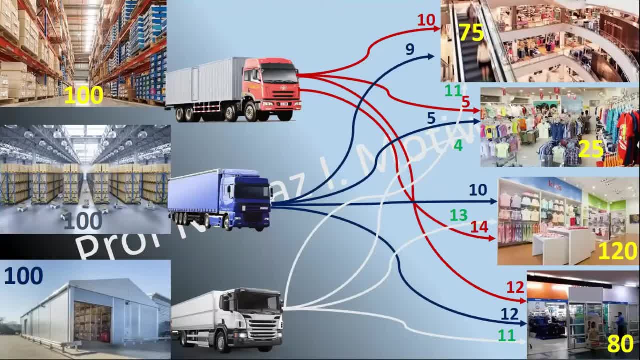 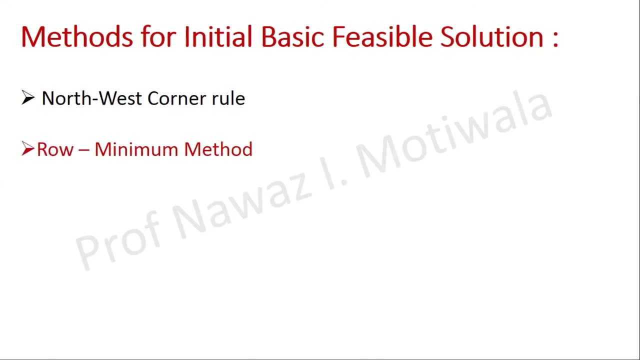 trouble and it will take a long time to solve what will be the optimum case or what will be the optimum units to be transferred to the various demand points from various warehouse. so there are some methods developed by our mathematicians to ease your calculation part, and these methods are. the first method is north west corner rule. next is the row minimum method. 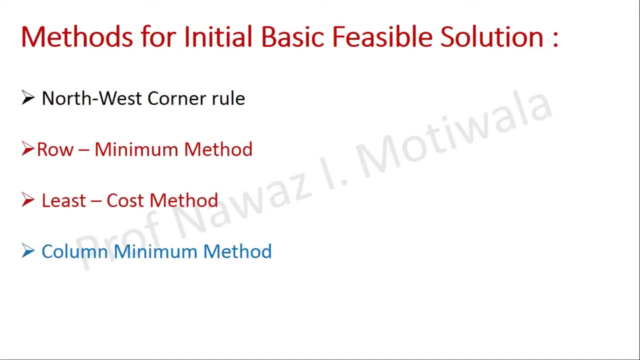 next will be least cost method, next is column minimum method and last one is vogel's approximation method. this method, the last one, vogel's approximation, is also known as penalty method or penalty cost method, and this is the method which is most probably, or most widely. 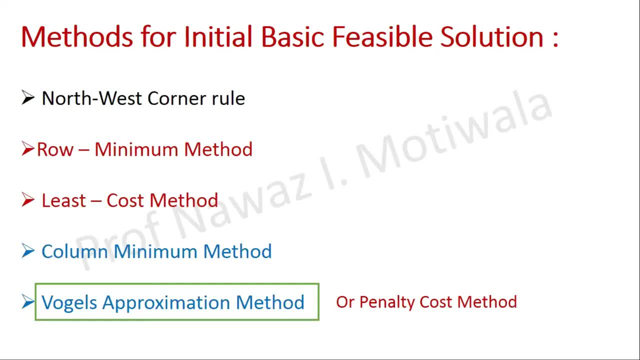 used. why? because it gives the solution very much near to the optimum. but we can rely more on vogel's approximation method for our solution in exam. also, if it is asked to find out: find initial basic feasible solution so you can go by any of the methods as mentioned above. north. 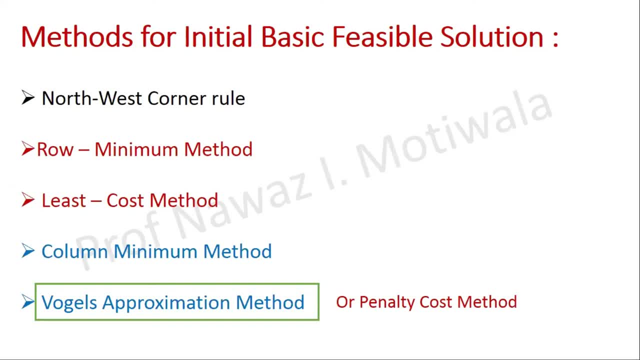 corner rule: row minimum: least cost, column minimum vogel's approximation: anything you can go, but it is advisable to go by vogel's approximation method because it gives the most closest answer. and why is it so we will see in the problems part. okay, so here you can see the heading is: 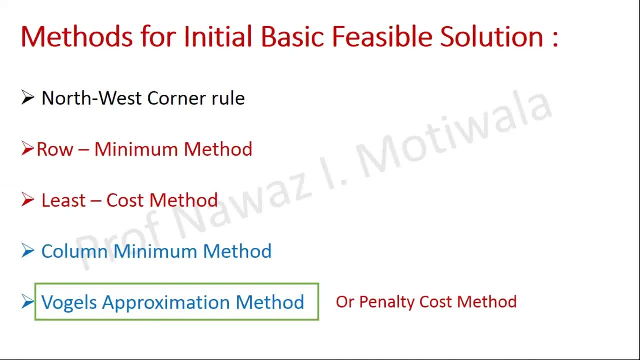 method for initial basic feasible solution. this, all methods, this all methods will just give you the basic feasible solution. it does not mean the solution found out by this methods are optimum. there can be some solution which is giving you the least cost. better than this, all five methods and.